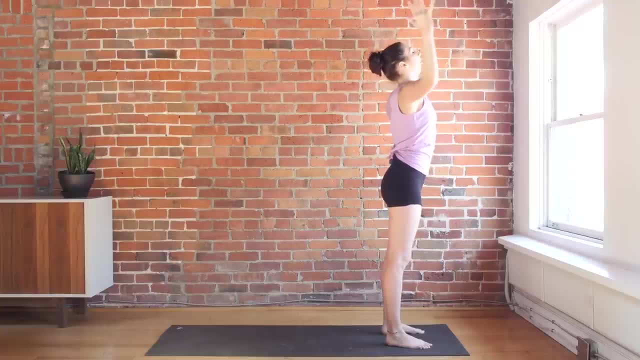 Big breath in through your chest and as you exhale round and contract, bring your arms back up, Bring your arms together and try to isolate this through your upper body, upper back. So inhale like cat and cow: Open up, Exhale round and pull it in One more, just like this. 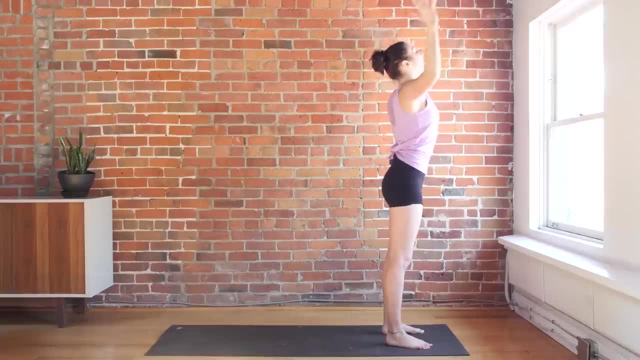 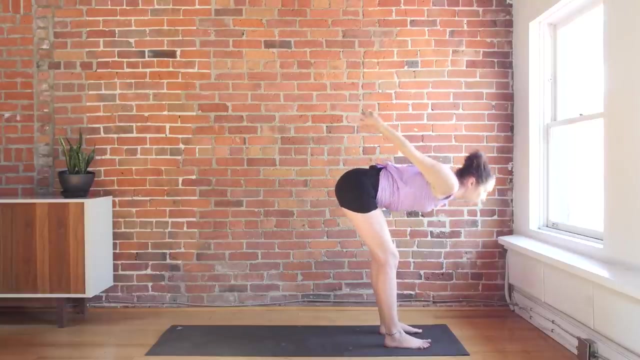 Inhale and exhale, Open your arms and interlace them behind your lower back. Roll your shoulders down and away from your ears as you inhale and inhale. Lift and look up and let's fold forward So you can definitely bend your knees here. 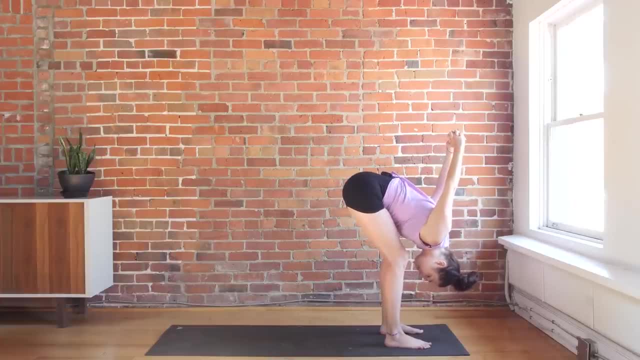 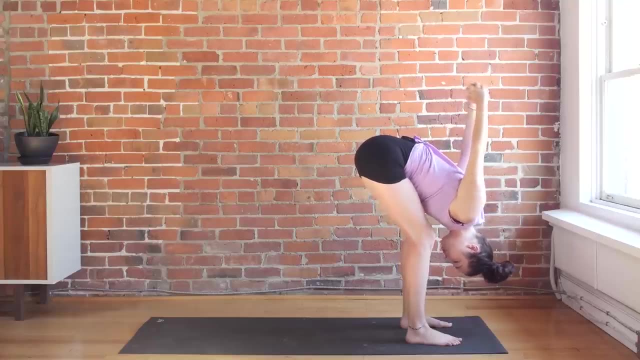 I like to bend my elbows a little bit so that I'm not locking them and hyperextending. And even though we're folding forward, see if you can lift your shoulders away from your ears and away from the floor. Let your head be even heavier Just lifting up through the knuckles. 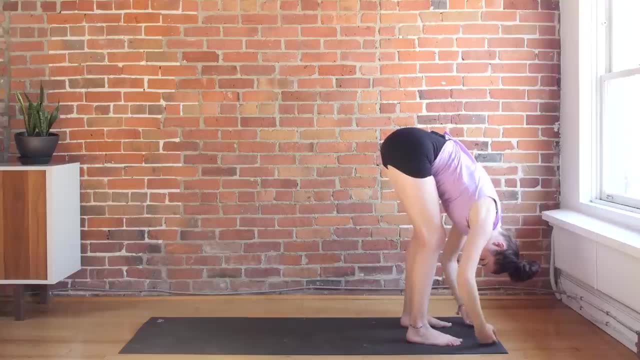 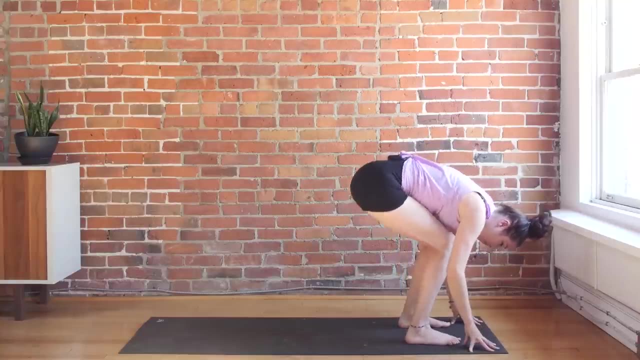 and stay in this forward fold. But just just let your arms and your hands relax down towards the floor And I'm going to come up onto the fingertips. We're just going to bend and stretch a few times, So bend into the knees and then go ahead and straighten the legs as you fold, Just warming up the hamstrings, Do that a. 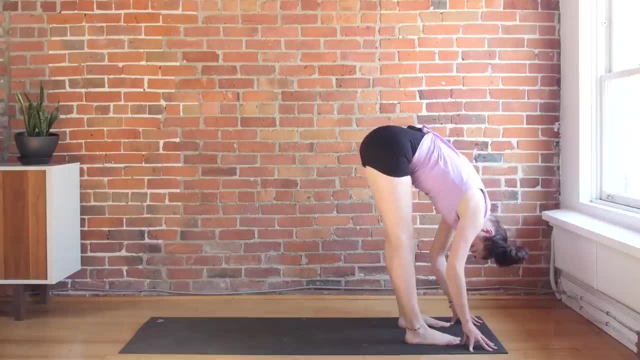 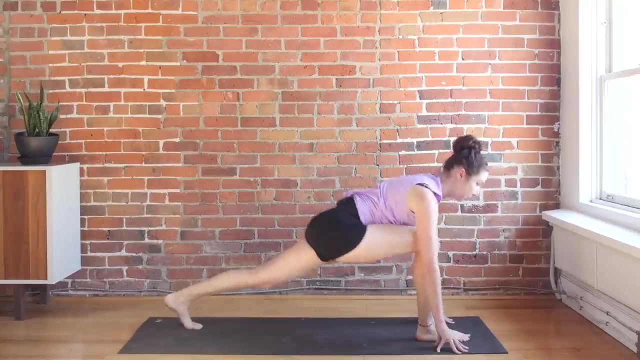 few more times. So morning flow is our opportunity to really set the tone for the day ahead, Putting yourself first, practicing some self-care and setting an intention that you can remind yourself of throughout the day. And bend a little into both knees- Just step your left foot back So you're in your runner's lunge. 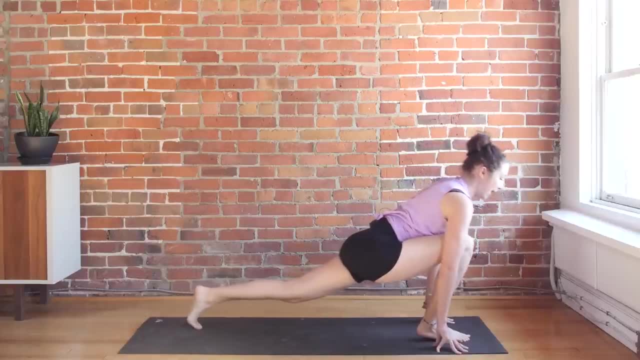 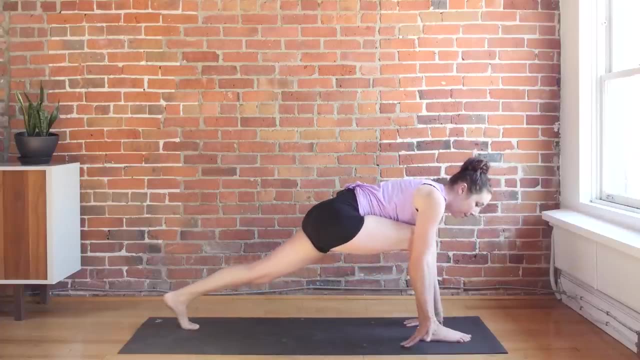 Back knee stays lifted and you might just wiggle a little bit back and forth If you'd like to stretch into your wrist. at the same time, you're going to turn so that your fingertips are pointing towards the back of the mat. Palms are flat to the floor. 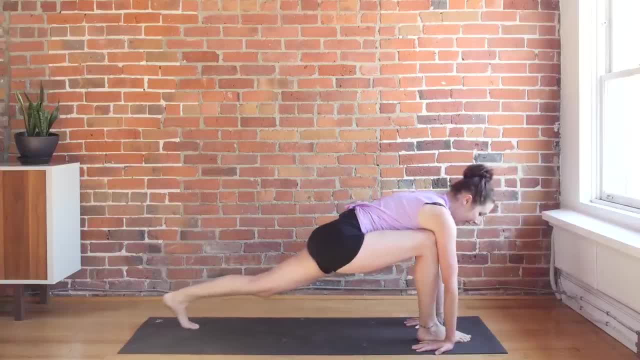 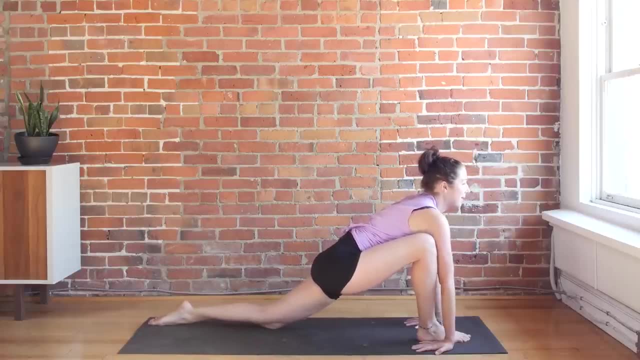 I'm just rocking a little back and forth. Go ahead and let your back knee come down to the mat, Stretching a little bit more into your forearms and into your wrists. You can start to push into your right heel a little bit. 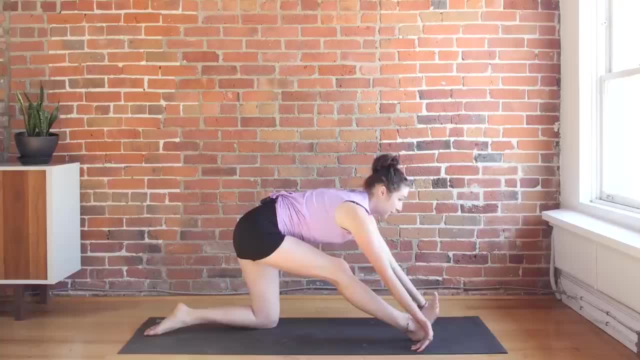 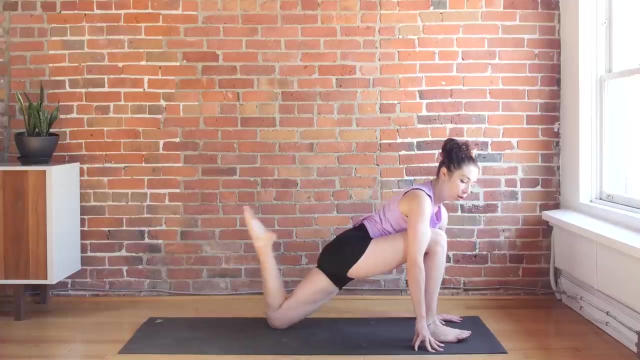 into your hamstring stretch and see if you can keep your fingers down On the mat. So just a different kind of wrist stretch And, coming back up onto fingertips, bend into your front knee again. Let's add a quad stretch. Bend into your back knee, Reach back with your right hand and see if you can pull your left. 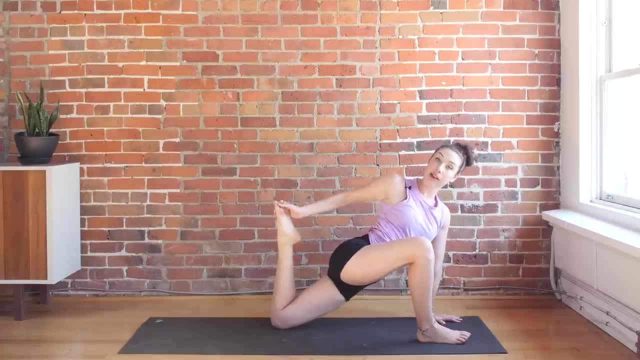 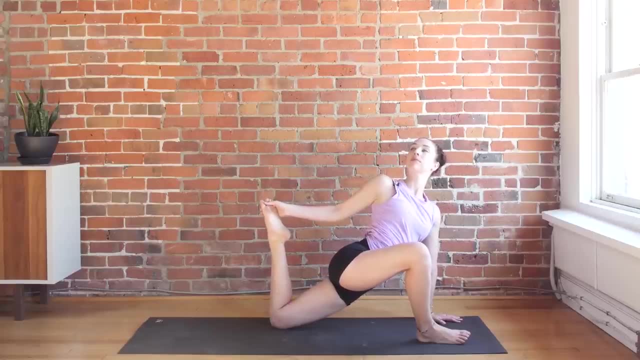 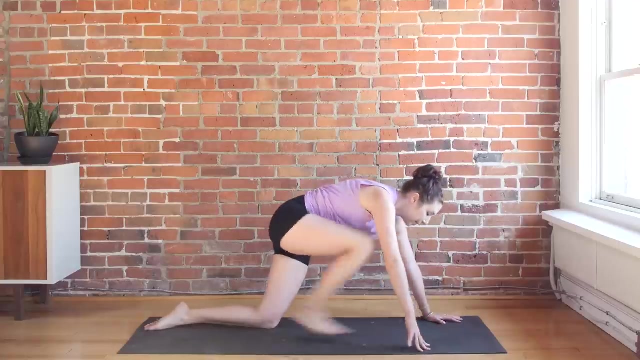 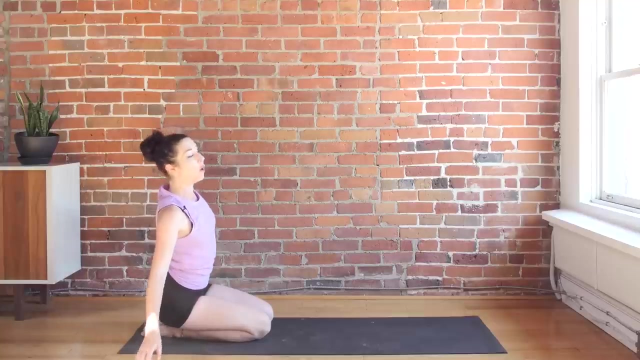 heel in towards you. So we're keeping our hips nice and low, rolling the right shoulder back, finding a nice lift. Carefully release the hold of your back foot And we're going to come back to kneeling. So both legs back behind you and sit your hips down onto your heels- A little side bend here. 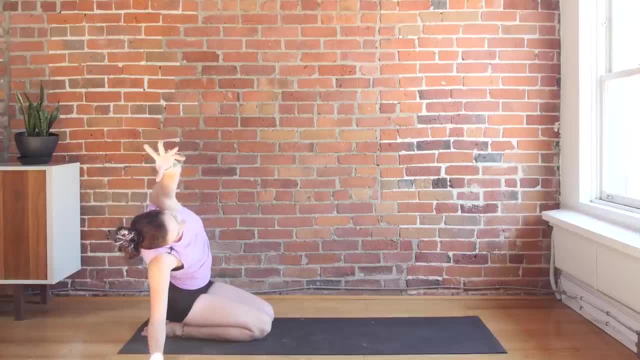 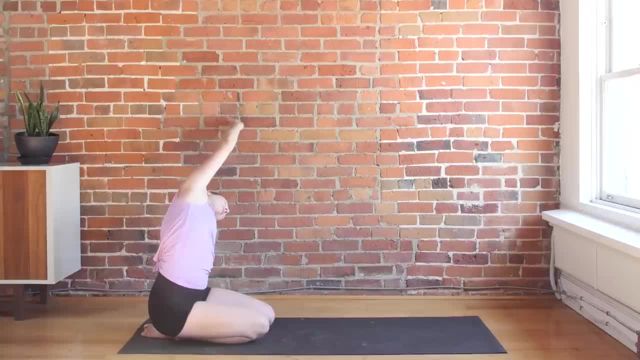 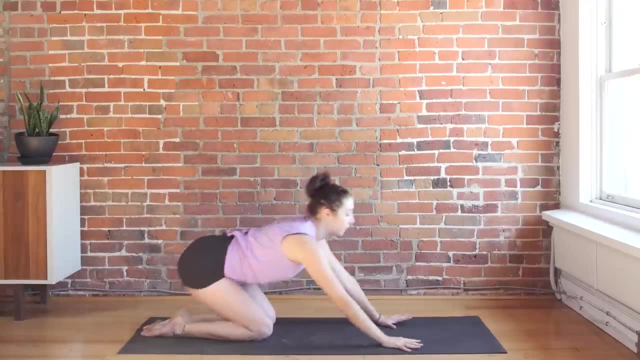 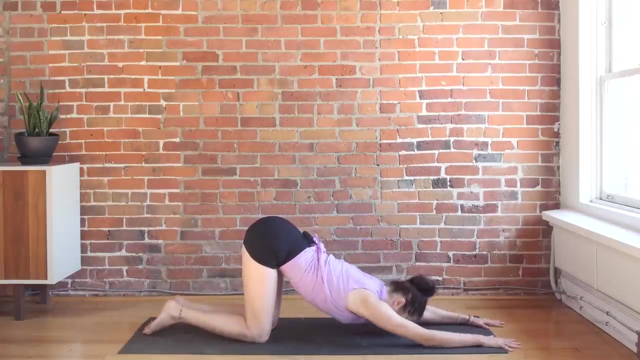 No tension, No tension in your jaw. Coming back through to center. Walk your hands forward, Puppy stretch, Keep your hips where they are over your knees and walk your arms out in front of you, Really working into the upper back. Take some deep breaths. 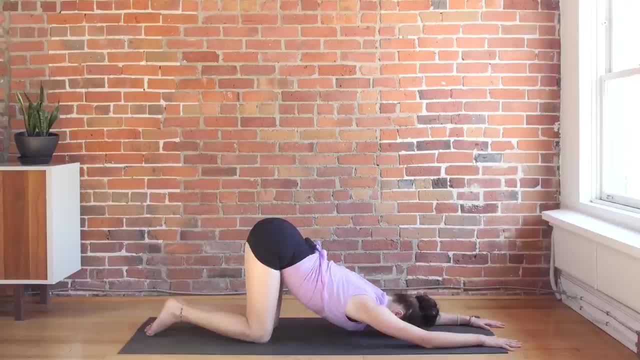 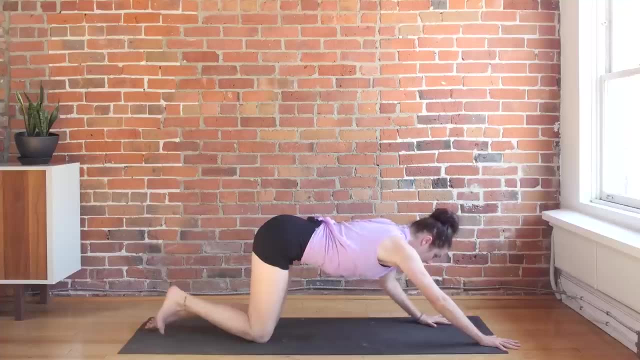 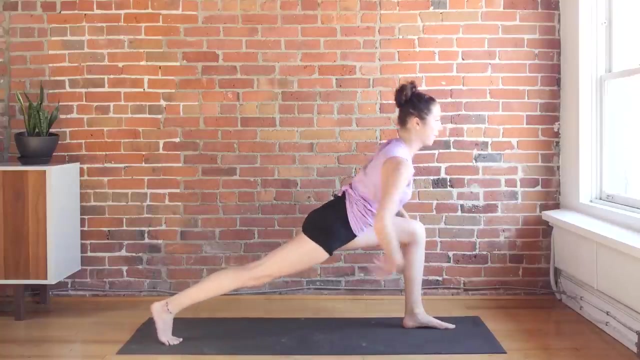 Go ahead and walk your hands in as you lift back up, Tuck your toes under, and we're just going to step our left foot forward to the top of the mat to finding your runner's lunge on the second side. So rocking back and forth This time. if you want to take a different, 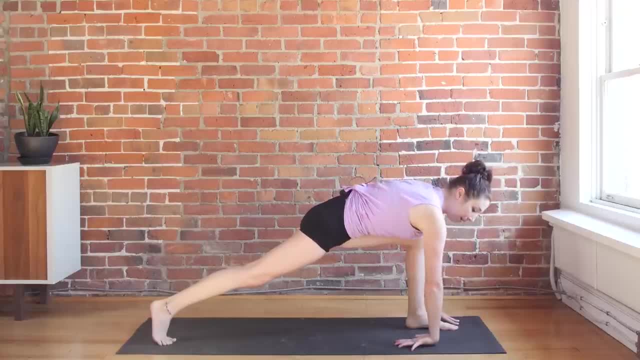 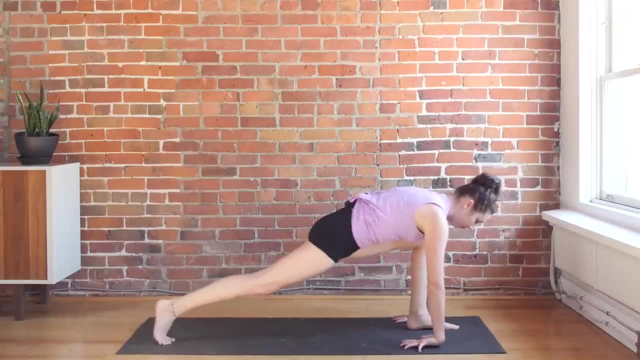 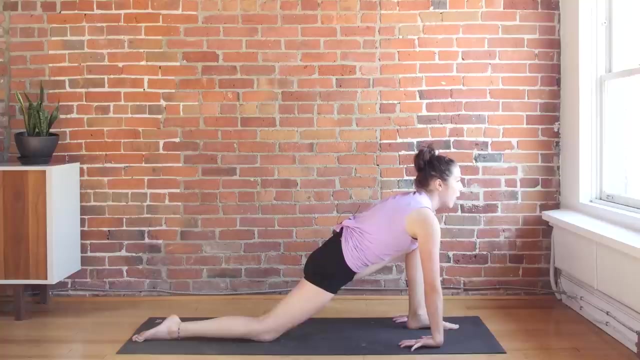 kind of wrist stretch. Again, the fingers point back, but this time bring the back of your hands on the mat. You might feel this more in one arm more than the other. Go ahead and ground that back knee to the floor, Finding a hamstring stretch. Try to keep the back of your fingers touching the mat. 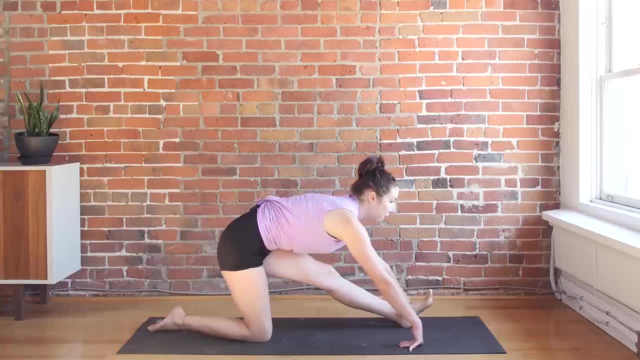 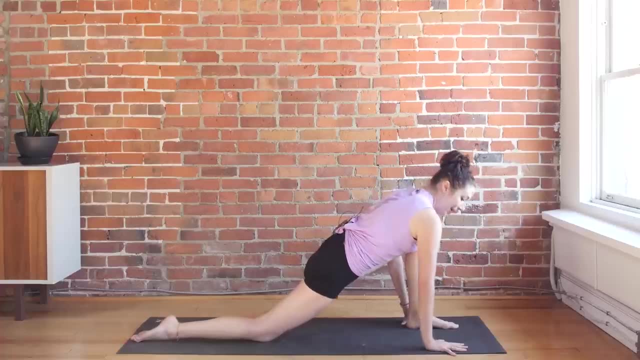 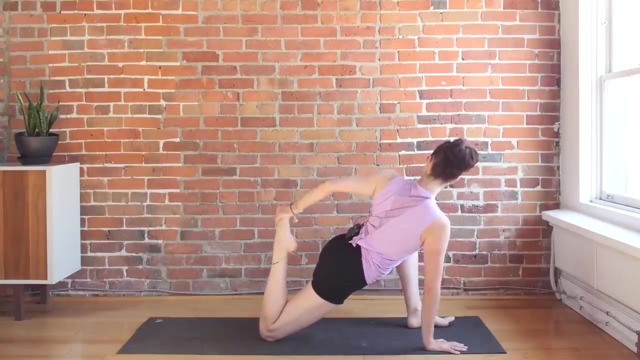 Stretch the hang, Reaching your heart forward. let's bend onto our forkquent knee and you're going to come question your watch. stretch here so you can let your right hand come flat to the floor. Reach back with your left hand, Grab ahold of your heel or your toes, whatever. 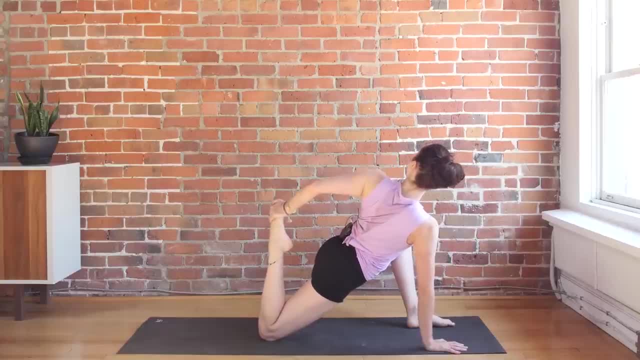 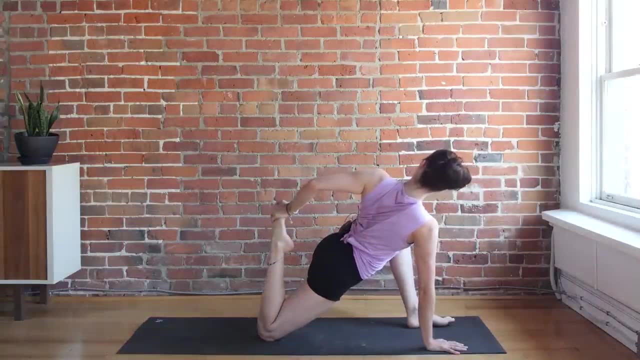 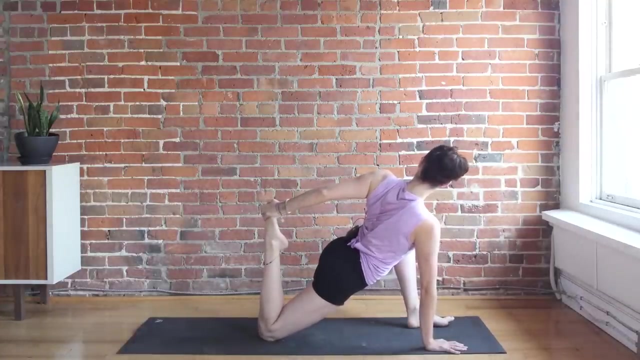 you can hold onto here, a little bit of a twist as we look over our left shoulder setting the tone for the day. What is one word, Etc? What is one word that captures how you want your day to go? One thing you want to focus on today: a feeling, an intention, maybe an action or a behavior. 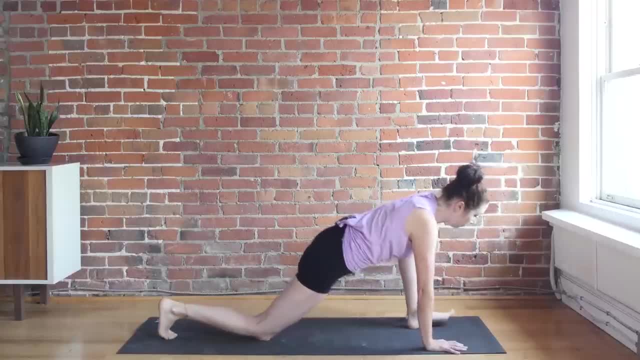 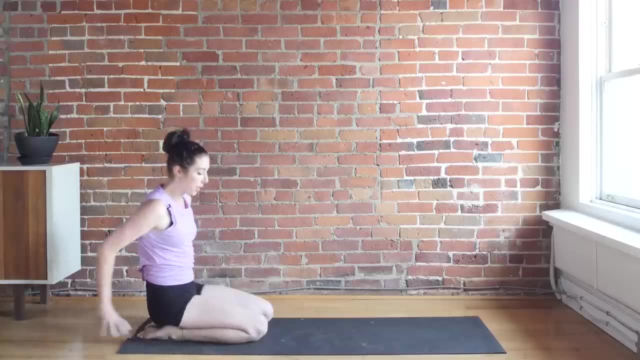 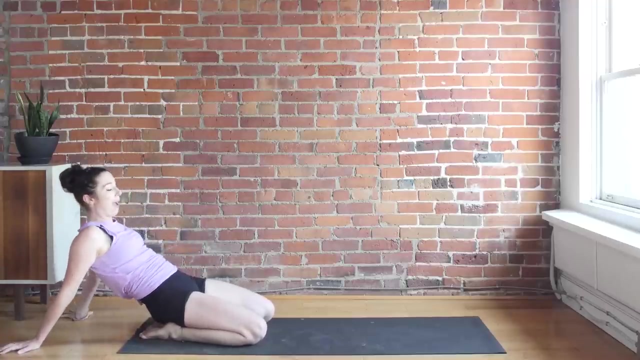 Carefully release that back foot and we're going to shift back kneeling once more, But this time, rather than going into our side body stretch, bring your fingertips back behind you, lift and tuck your tailbone under and you might just walk back a little bit. 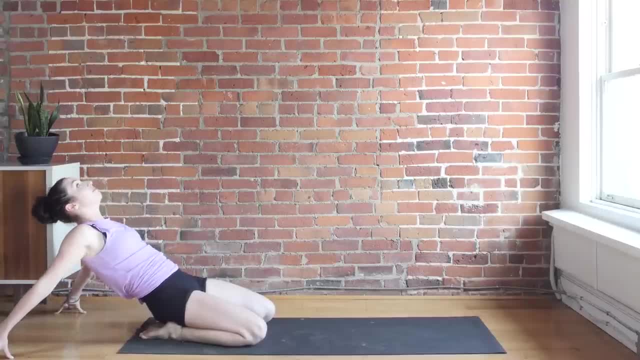 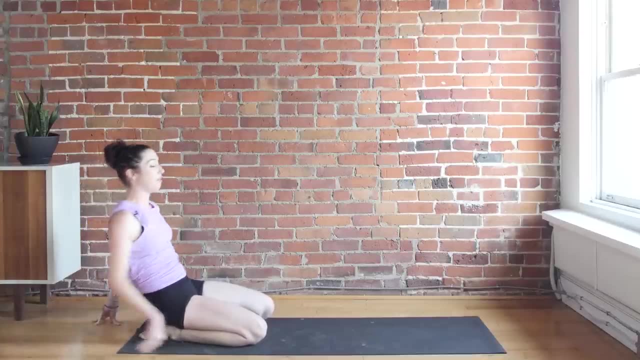 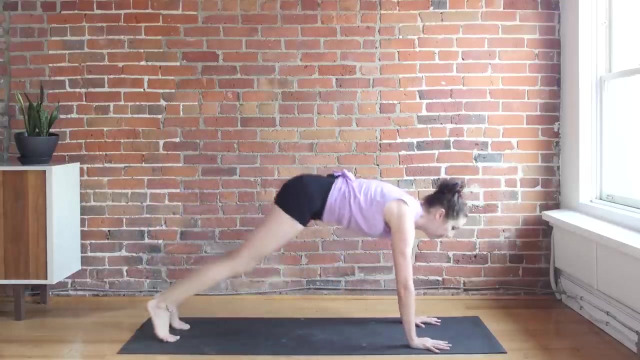 stretching into your quads a little bit further And lifting all the way back up. instead of going into puppy pose, let's find our full downward facing dog. Hands are shoulder width distance apart. feet are hip width distance apart. tuck your toes. 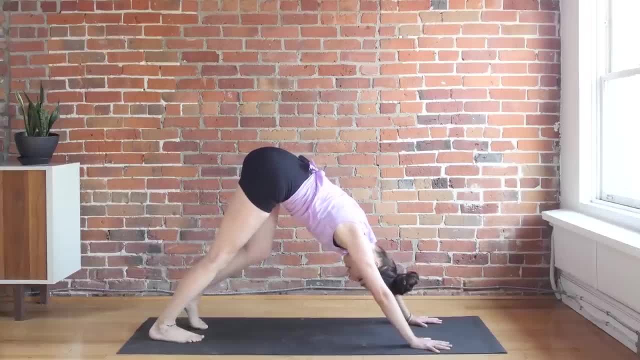 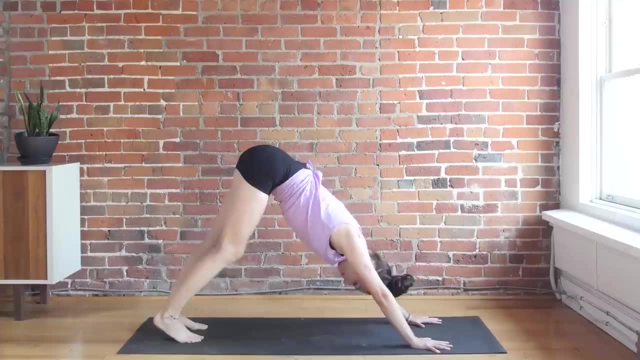 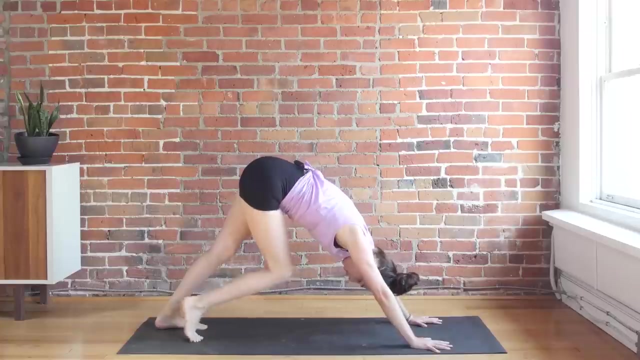 under and lift your hips up and back And you can paddle your feet here, maybe swaying a little through your hips. try to get the creases of your elbows to spin and rotate so they're facing forward, towards the top of your mat. 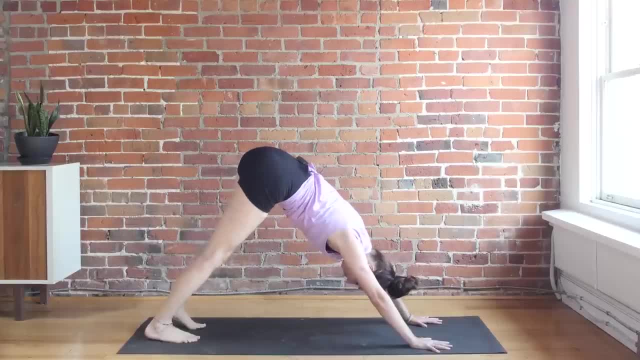 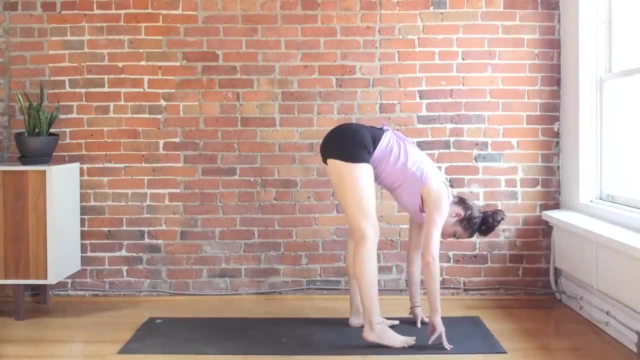 So there's an external rotation through your shoulders. Let's walk our feet to the front of the mat again, into your ragdoll fold. This time grab ahold of your elbows. You can let your knees bend. You can bend a little bit as you sway side to side. 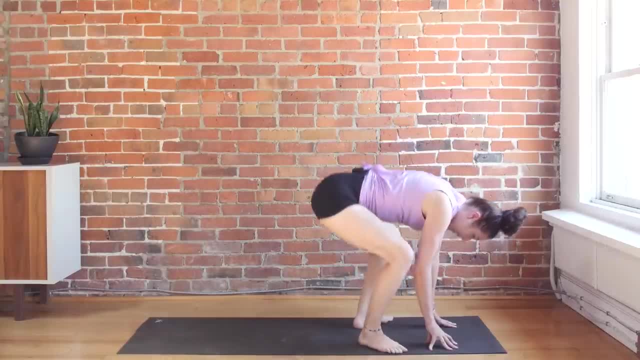 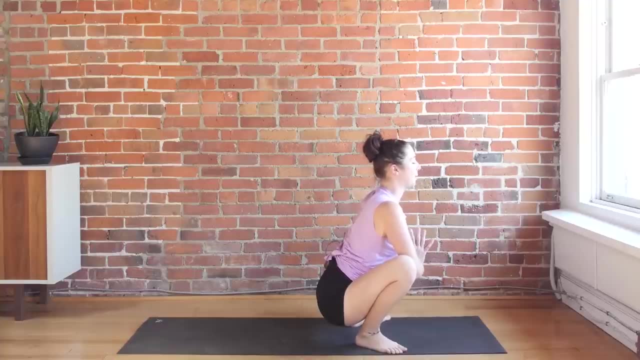 Into your yogi squat malasana: heels in, toes out. Sink it down low. Press your hands to your heart. use your elbows to push your knees and your thighs away from each other. Reach the crown of your head up towards the sky. 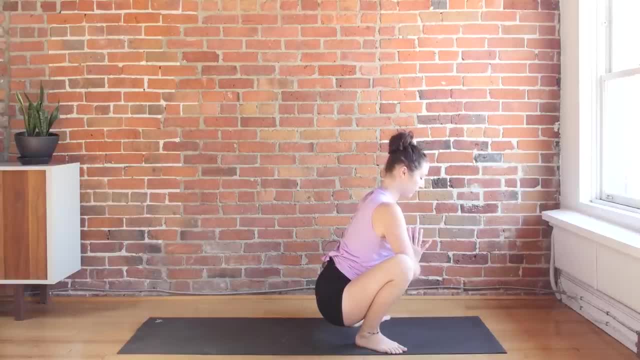 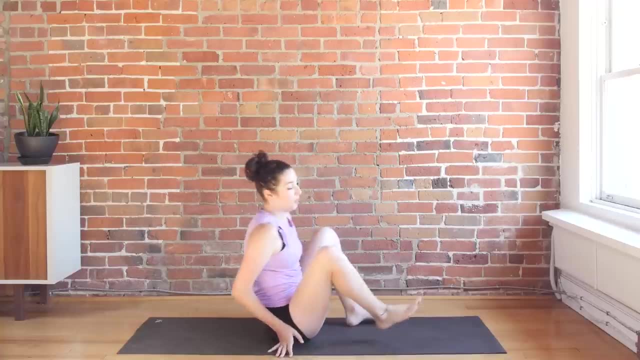 And we'll come into a pose- star pose, I've heard it called a few different things actually. So very similar to a butterfly forward fold, but instead of having your soles of the feet together, widen your feet and flex your feet. 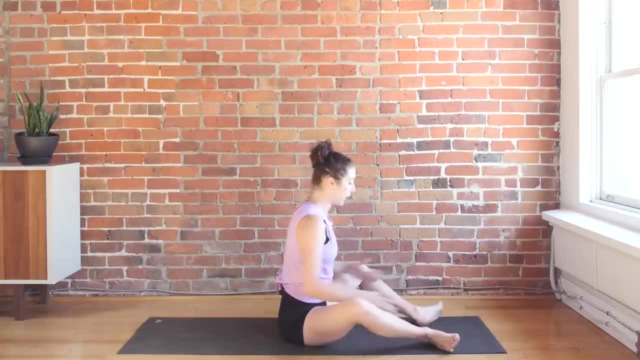 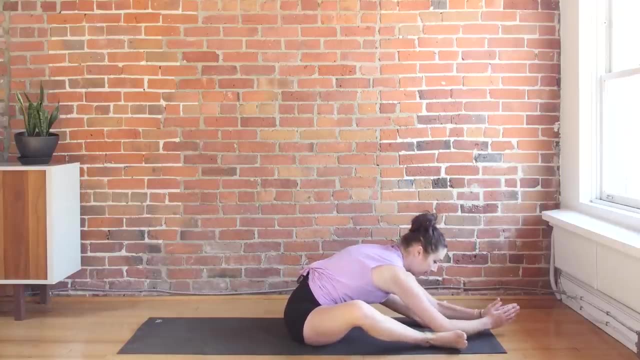 So you want to have about six inches or so between your heels and your feet aren't quite close to you And let your knees fall apart from each other And then start to initiate the fold. And then start to initiate the fold- And I like to let my spine round, naturally, here, minimizing any tension or effort. 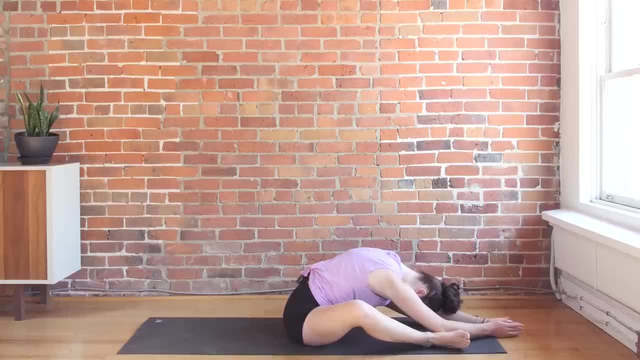 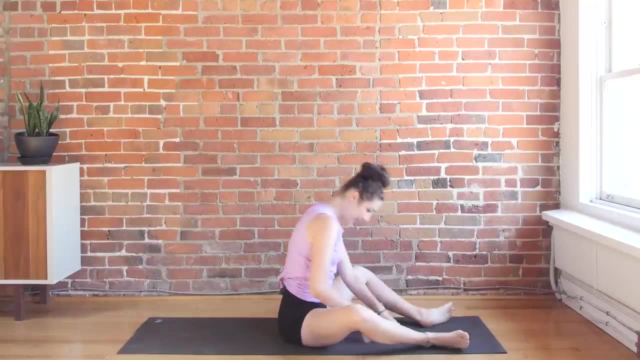 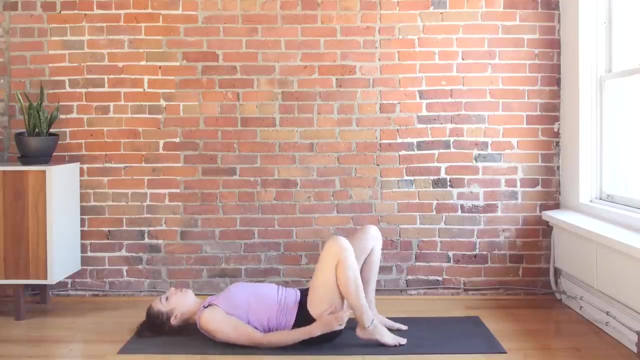 Coming all the way back up. Let's lay down on our backs. keep your feet flat on the floor. knees are bent. roll your shoulders down and away from your ears into your bridge pose. inhale, push into your feet, lift your hips up, squeeze through your inner thighs. 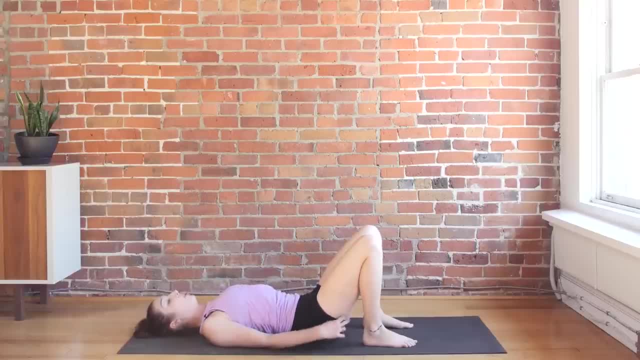 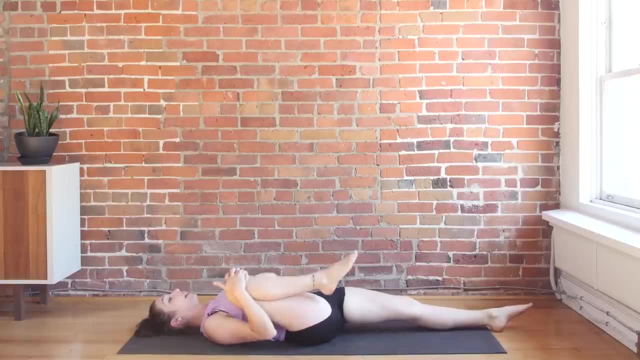 exhale slowly, lower down, pull your right knee in towards your belly and go ahead and straighten your left leg to the floor so right knee pulls in and we'll carry it over into a twist so you can cross your right knee over your body to the left and maybe your right arm extends out to the side. 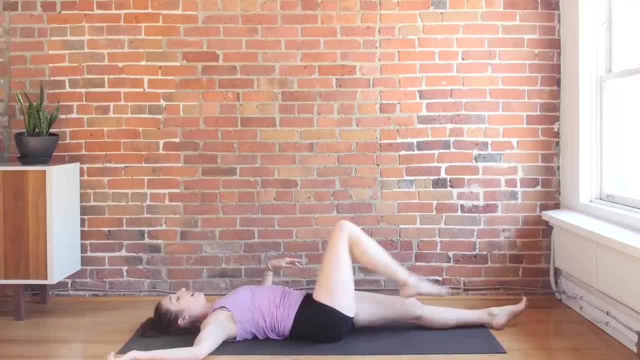 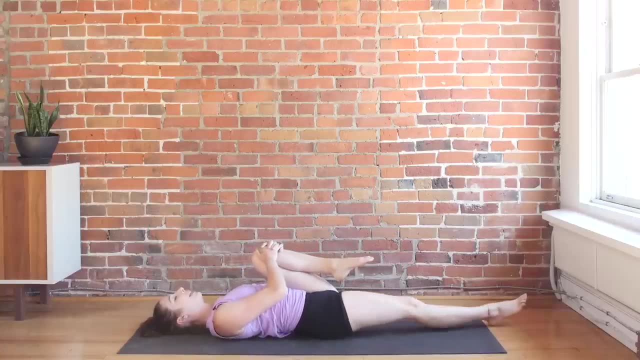 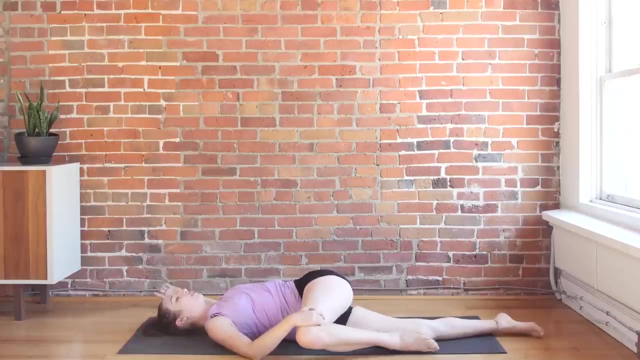 So come on Coming back through to center, let's switch sides. right leg is straight. left knee bends as you draw it in towards your belly. Maintain this length. even as you twist, carrying your left knee over towards the right side of your mat, left arm reaches out. 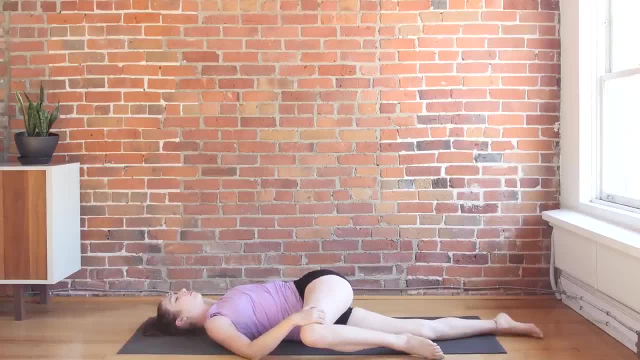 Maintain this length. even as you twist, carrying your right knee over towards the right side of your mat, left arm reaches out. Maintain this length. even as you twist, carrying your left knee over towards the right side of your mat, left arm reaches out. 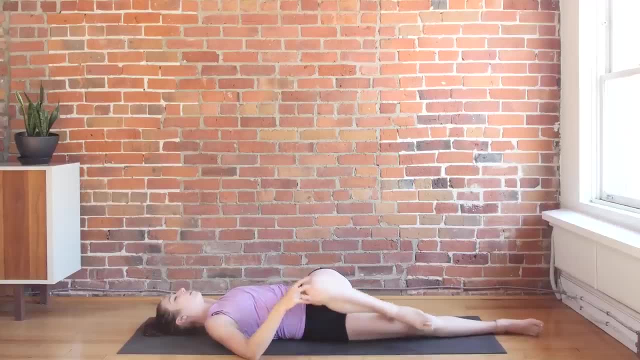 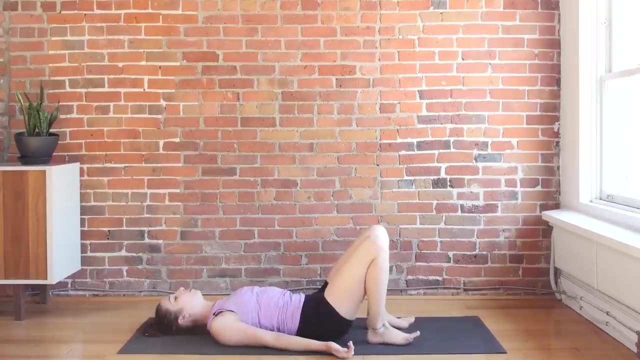 Coming all the way back through to center. bend your knees again. we're going to find our bridge pose one last time: feet flat to the floor. Push your feet into the floor, squeeze and lift all the way up. Hug in.